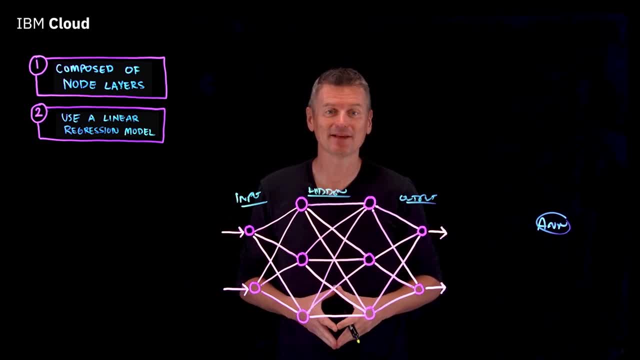 And so out of the artificial neural network there is a know-how到 ajuda that will become known in the used computers, ancercognition models. you can get a handle on how to calculate. the weight provides you with all these examples and The weights of the connections between the nodes determines how much influence each input. 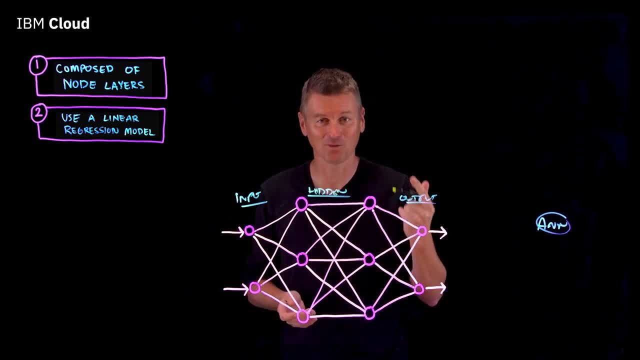 has on the output. So each node is composed of input data, weights, a bias or a threshold, and then an output. Now data is passed from one layer in the neural network to the next in what is known as a feed forward network. number three: 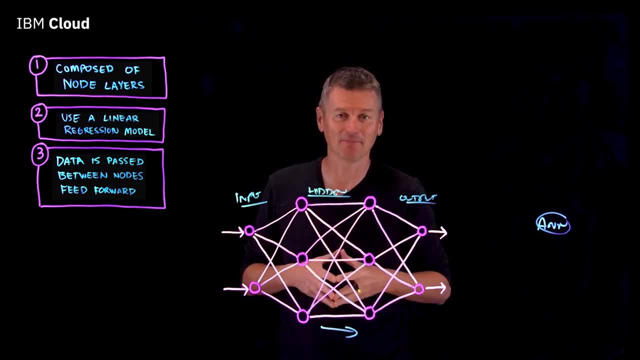 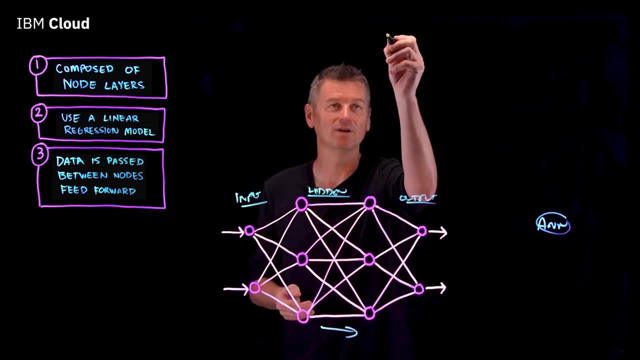 To illustrate this, let's consider what a single node in our neural network might look like to decide should we go surfing. The decision to go or not is our predicted outcome, or known as our Y hat. Let's assume there are three factors influencing our decision. 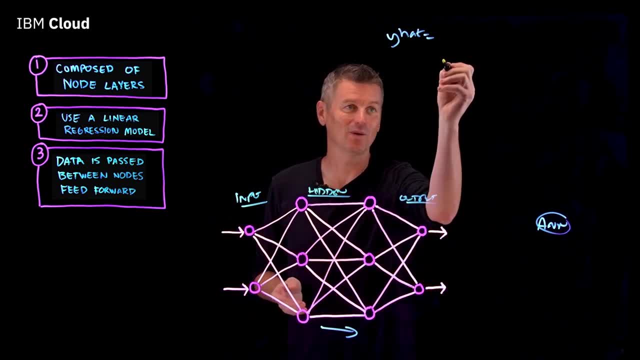 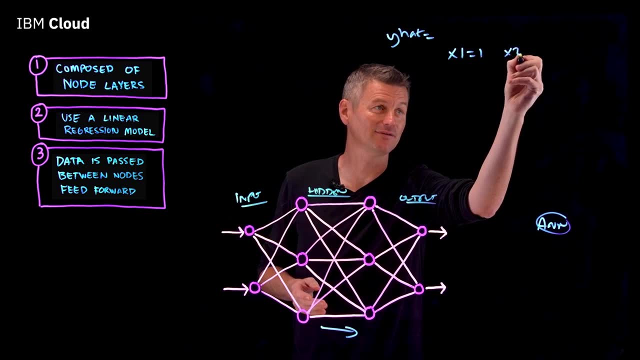 The waves. good one for yes or zero for no. The waves are pumping, so X1 equals one, one for yes. Is the line up empty? Well, unfortunately not, so that gets a zero. And then let's consider: is it shark free out there? 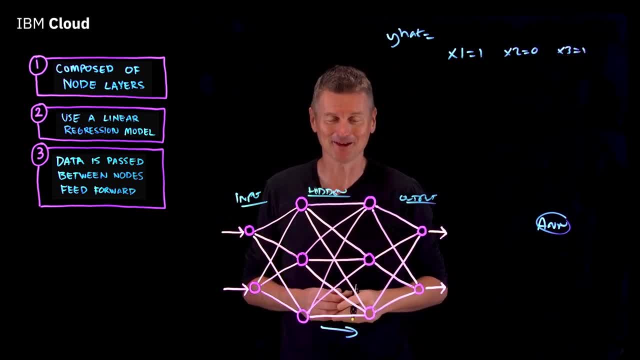 That's X3.. And yeah, no shark attached. Okay, This is a free shark. So what do we get? We get an X3.. We get a zero, We get an X3.. So what is the difference between the waves and the sharks? 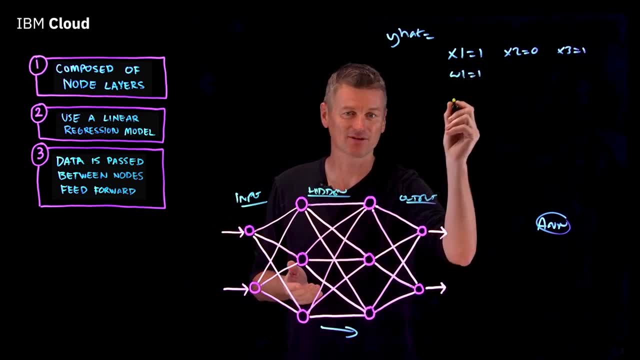 Well, the way to get that is by simply adding a gradient to that gradient, As this you can see here we'll write the Gracias to 0.. We're going to give that a 3.. And so we get a 2.. 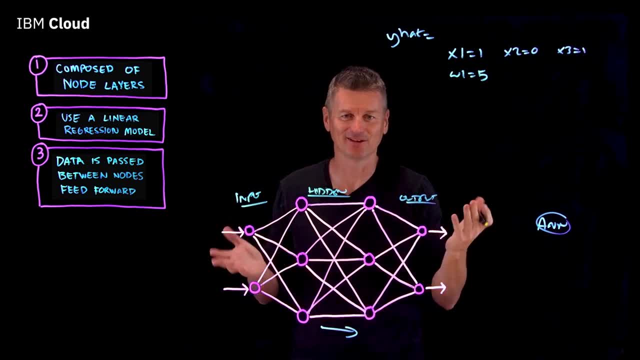 And this one is a 4.. And this is also an X. We're going to make a little bit more clear about this. We're just going to put down our first graph here. We're going to take this to the left. We're going to take this to the right. 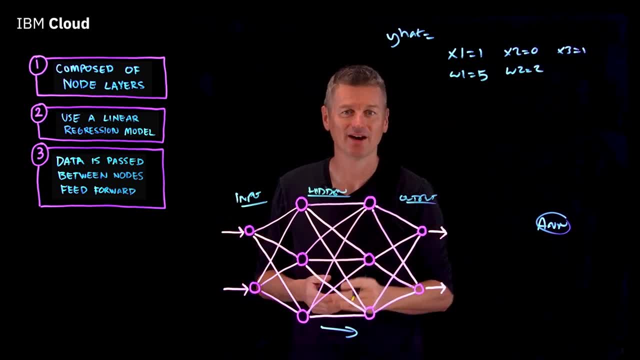 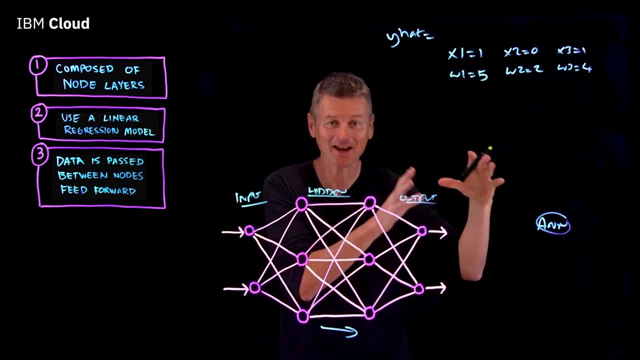 And if we want to have the first graph we're going to put down- here's the first graph- we're going to take the third graph, important, we'll give that a 2.. And sharks: well, we'll give that a score of a 4.. Now we can plug. 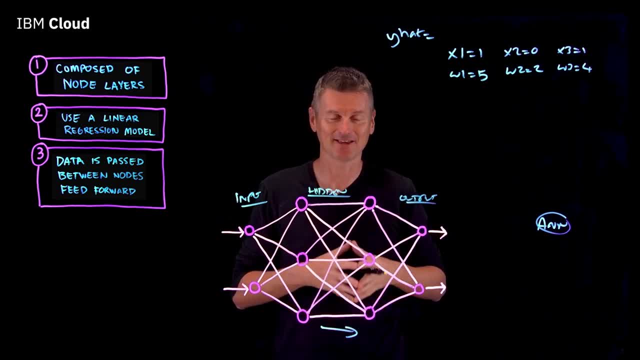 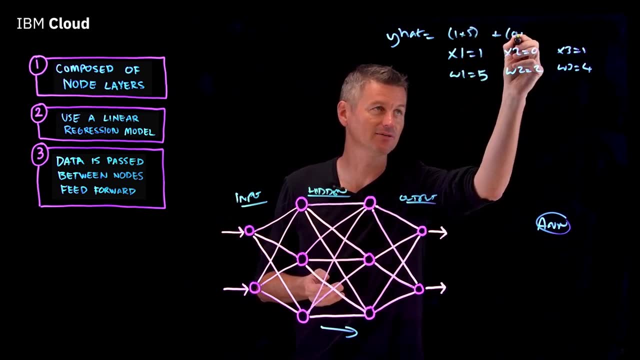 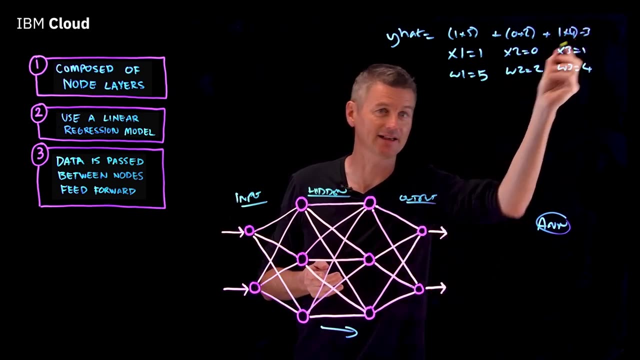 in these values into the formula to get the desired output. So y hat equals 1 times 5 plus 0 times 2, plus 1 times 4, then minus 3, that's our threshold and that gives us a value of. 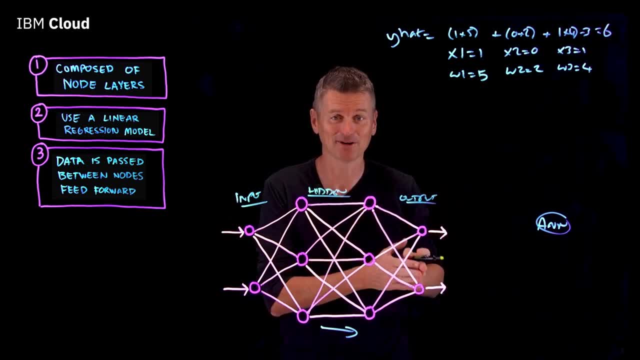 6. 6 is greater than 0, so the output of this node is 1.. We're going surfing, And if we adjust the weights of the threshold, we can achieve different outcomes. Number 4. Well, yes, but 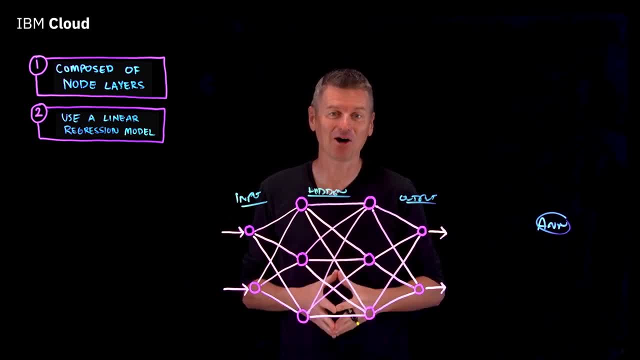 of the connections between the nodes determines how much influence each input has on the output. So each node is composed of input, data, weights, a bias or a threshold, and then an output. Now data is passed from one layer in the neural network to the next in what is known as a feed forward network, Number three to. 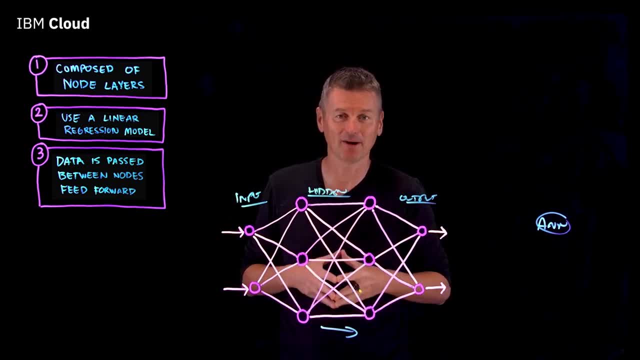 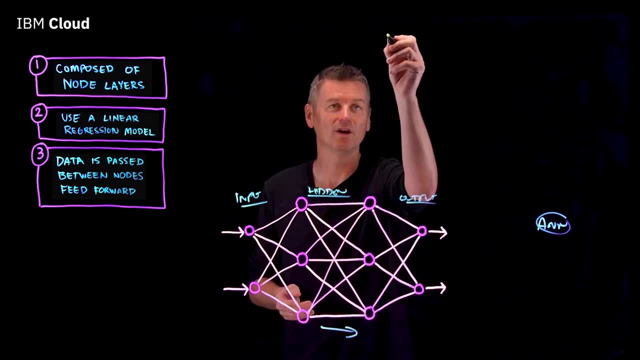 illustrate this. let's consider what a single node in our neural network might look like to decide should we go surfing. The decision to go or not is our predicted outcome, or known as our y-hat. Let's assume there are three factors influencing our decision. Are the waves good? 1 for yes or 0 for no? The waves are. 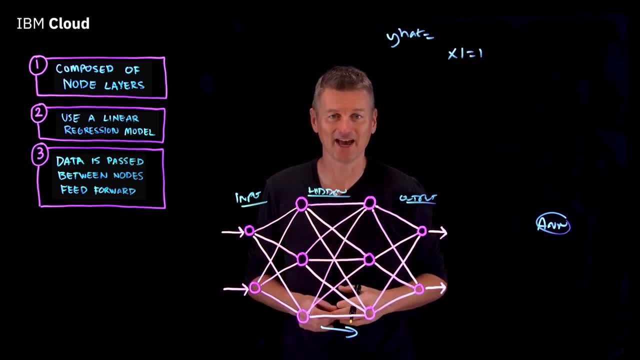 pumping. so x1 equals 1,, 1 for yes. Is the line up empty? Well, unfortunately not, so that gets a 0.. And then let's consider: is it shark free out There? that's x3, and yet no shark attacks have been reported. Now to each. 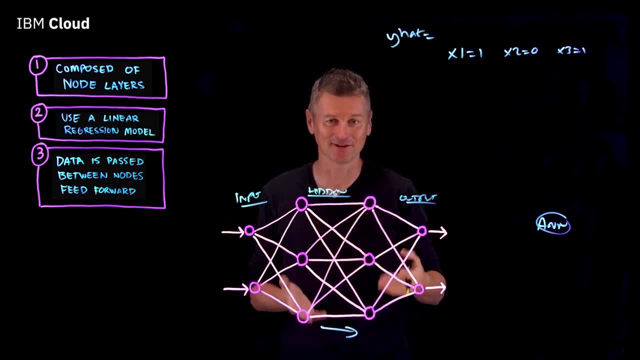 decision, we assign a weight based on its importance on a scale of 0 to 5.. So let's say that the waves we're going to score that one, yeah. no, this is important, let's give it a 5.. And for the crowds, that's w2, yeah, not so important, we'll. 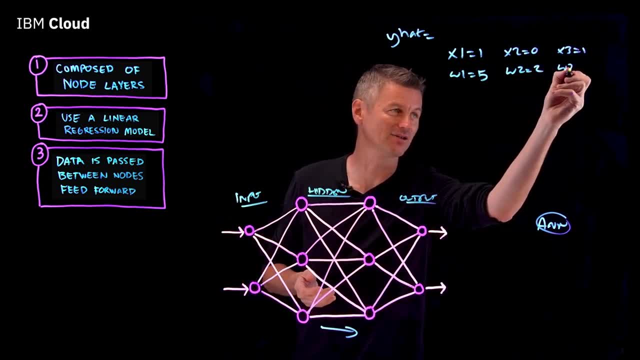 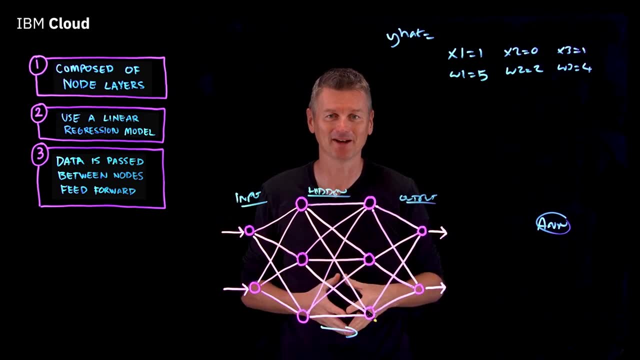 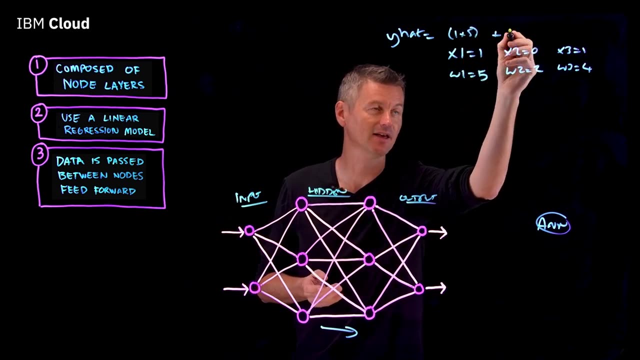 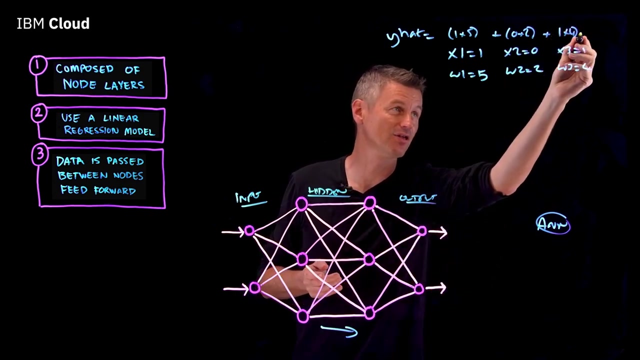 give that a 2.. And sharks, well, we'll give that a score of a 4.. Now we can plug in these values into the formula to get the desired output. So y-hat equals 1 times 5 plus 0 times 2, plus 1 times 4, then minus 3, that's our threshold and that 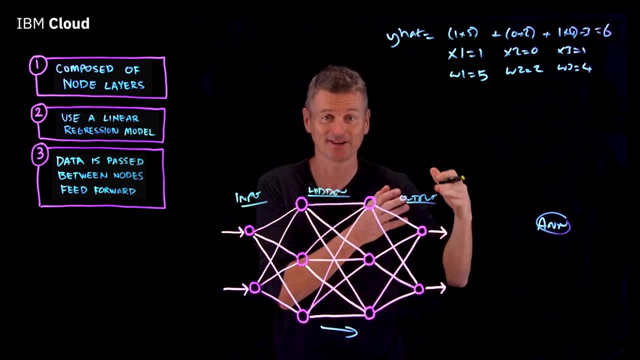 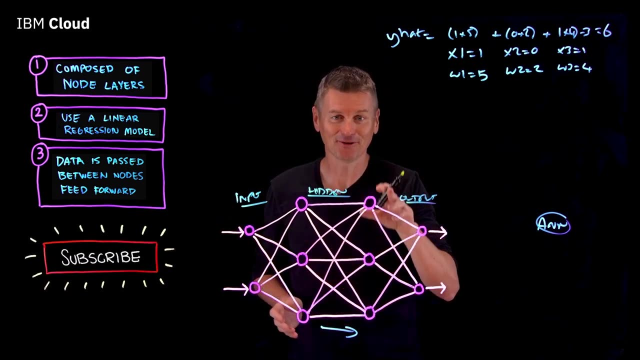 gives us a value of 6.. 6 is greater than 0, so the output of this node is 1.. We're going surfing, And if we adjust the weights of the threshold, we can achieve different outcomes. Number four: Well, yes, but number four: Neural networks rely.